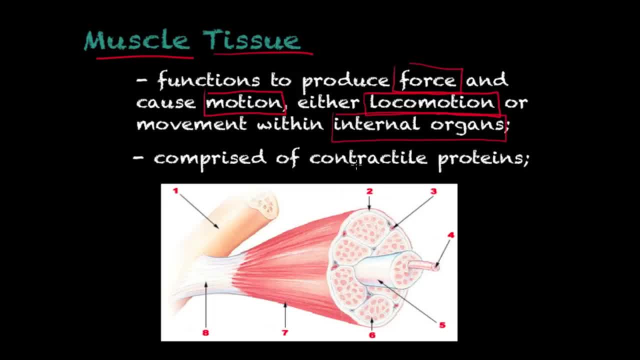 Now, the second thing that I want to tell you- and it's a very important, key thing about muscle tissue cells, is that they are comprised of what they call contractile proteins, And these are special types of proteins called. they are actin and myosin, And these two form 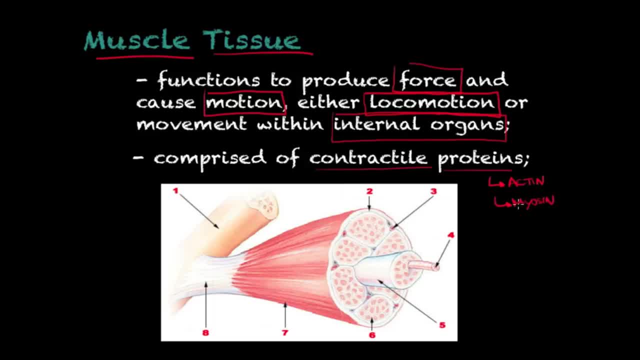 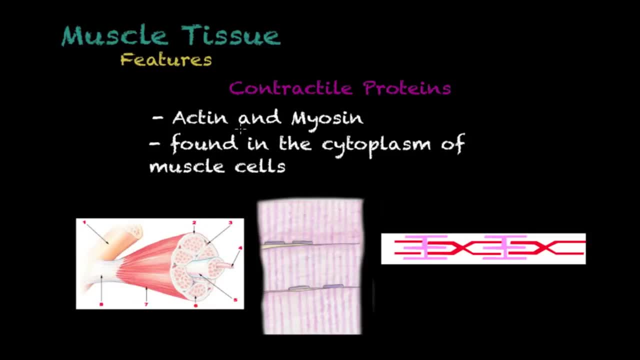 a special device, let's say, which allow the cell to contract and therefore produce the movement that we have been talking about. So I would like to go into the features or the characteristics of muscle tissue cells, and one of the things that I already mentioned is that they are contractile. 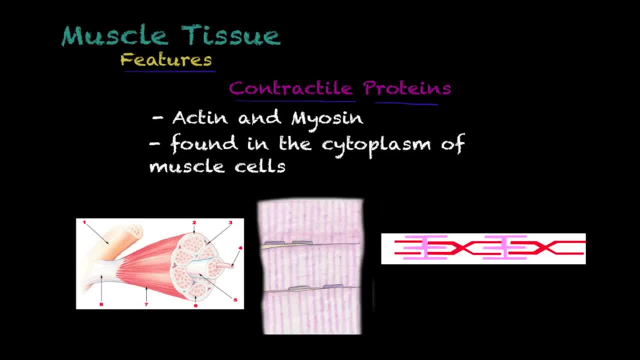 or they have contractile proteins, And these contractile proteins are actin and myosin, and they are found in the cytoplasm of muscle cells. Now, if I want to show you this in a little bit more detail, I have three pictures that will illustrate this. And the first one. 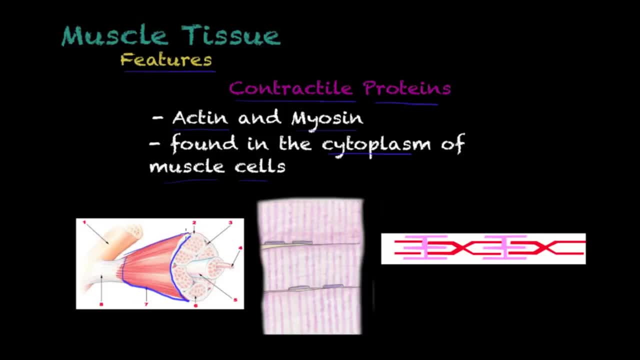 a macroscopic view of a muscle and then, if I go into a little bit more detail here until I can get into microscopic view of the actual cell, I have a muscle tissue cell or a muscle cell here where I can see nuclei and one of the very 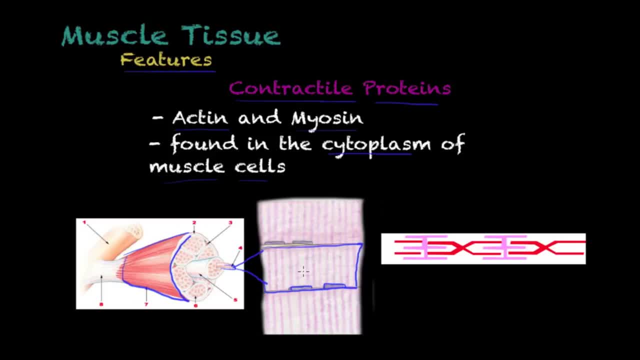 interesting characteristics of muscle tissue cells or muscle cells is that under a microscope they have these lines called striation and they are caused by these actin and myosin fibers or proteins. they are able to cause this striation. here now what I want to also show you in more detail. say, if you want: 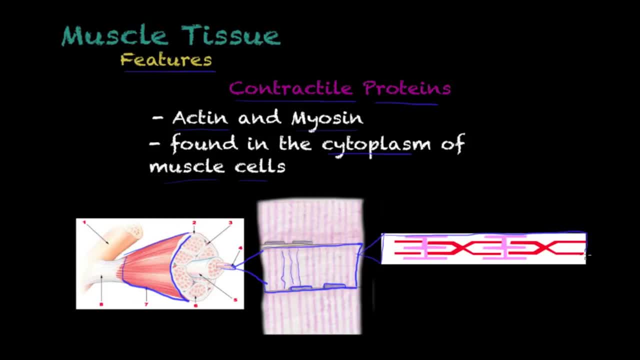 to look under an electron microscope, you will see a structure that looks a little bit like this, and it's formed by actin and myosin. yeah, It's called a sarcomere, And what this is is my red here is representing myosin. 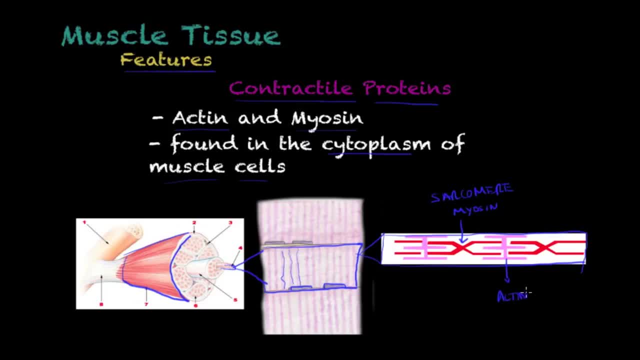 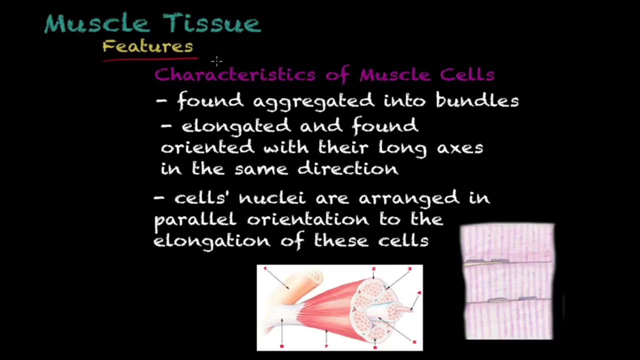 And the pink here is actin filaments. So and what happens here is when these fibers or these proteins move along one another, they can cause contraction. So I would like to add some more characteristics or features of muscle tissue cells. One of them is that these cells are found aggregated into bundles. 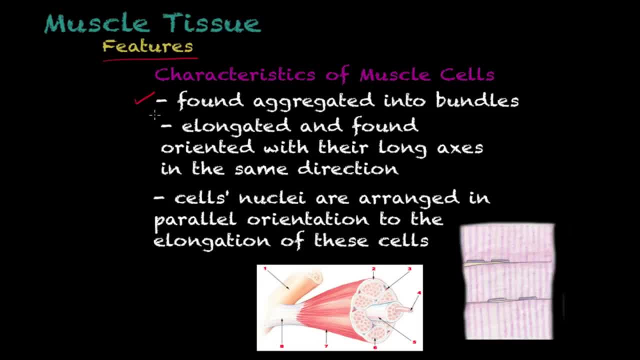 This is the only way muscle tissue is able to actually produce movement, because these cells work in groups. Another thing that is important to mention is that these cells are elongated, meaning if I look here at my cells illustration, here They are elongated or long cells. 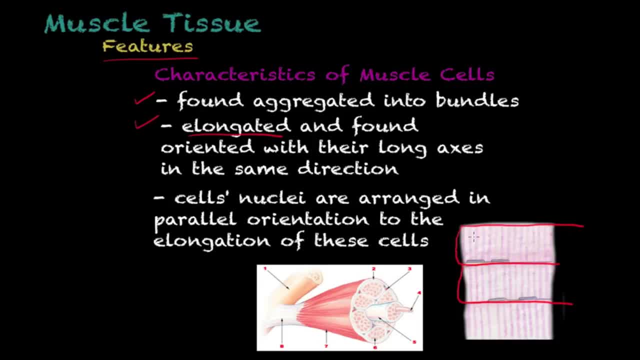 And they are oriented with their long axis in the same direction. So these cells are oriented in the same direction. Also, the nuclei of these cells are arranged in parallel orientation to the elongation of these cells. So if they are elongating this way, the nuclei, as you can see here, is going to be found. 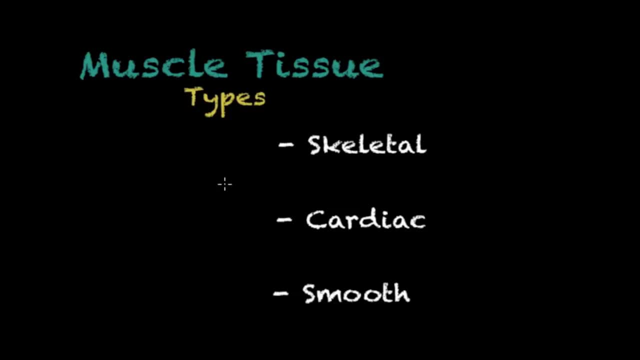 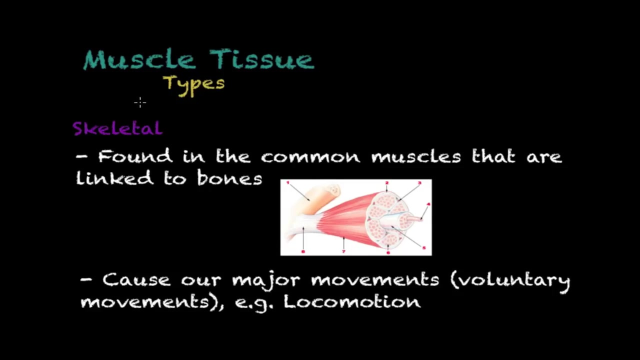 in this manner. There are three types of muscle tissue and we are going to briefly, briefly discuss them. The first one is skeletal muscle, cardiac muscle and smooth muscle. So the first type of muscle tissue that I would like to briefly discuss is skeletal muscle tissue. 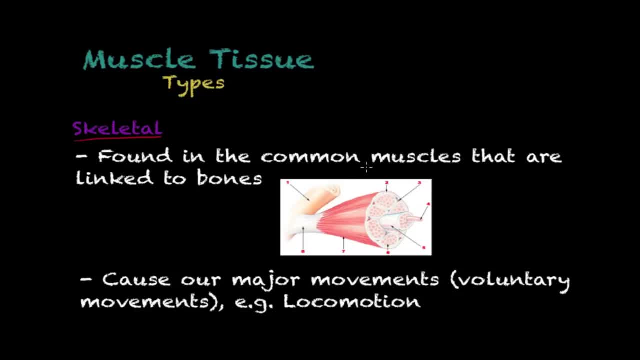 And this is the type of tissue that you find in the common muscles and that are linked to bones. These, This tissue causes the major movements, voluntary movements. An example of that is locomotion. When you walk, for example, you are using your major muscles and your major muscles. 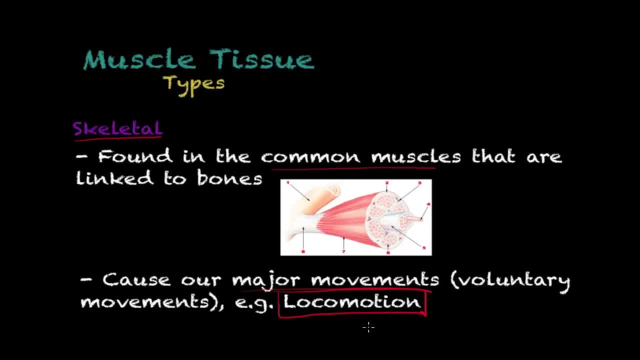 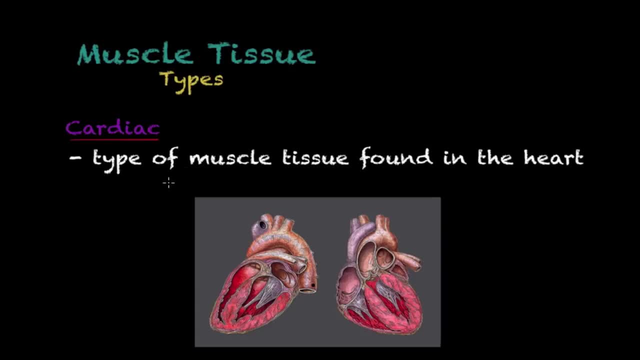 of course, are comprised of skeletal muscle tissue. Another type of muscle tissue is cardiac And, as the name indicates, this is the type of muscle tissue that you find in the heart. It is Thanks to this muscle tissue that the heart is able to contract and pump blood all over. 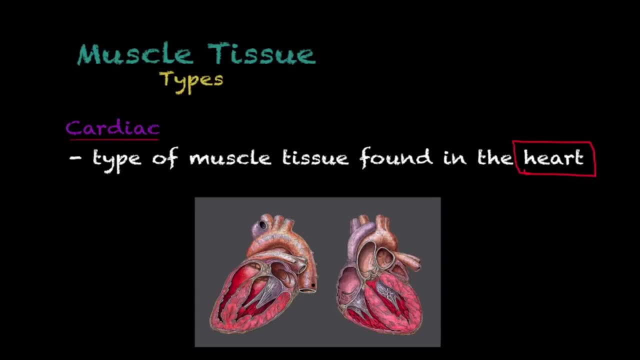 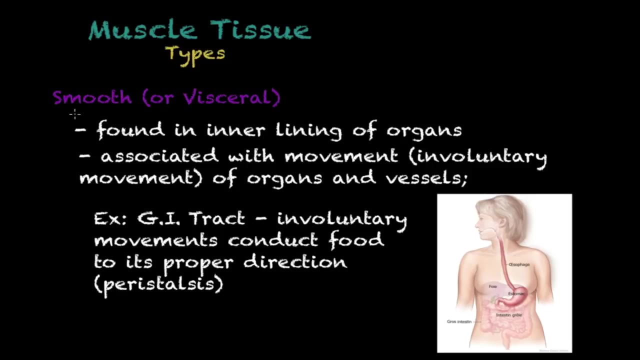 your body. So, as you can see, this heart here, or the heart, is comprised of mostly muscle tissue, which is then able to perform that function. So this is the last slide of this lecture where I am going to talk about smooth muscle. tissue, Also known as visceral muscle tissue. So this is the last slide of this lecture where I am going to talk about smooth muscle tissue, Also known as visceral muscle tissue. So this is the last slide of this lecture where I am going to talk about smooth muscle tissue. 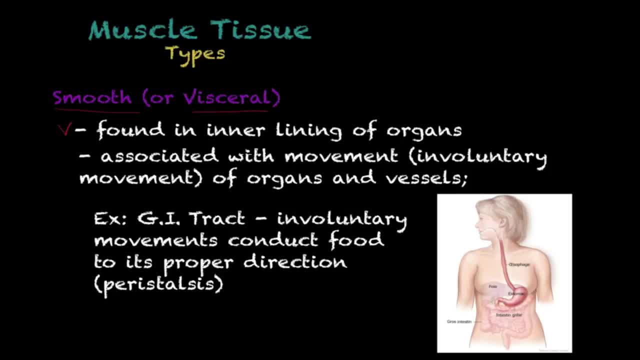 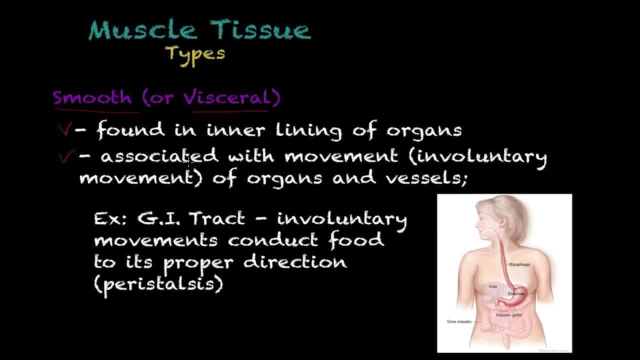 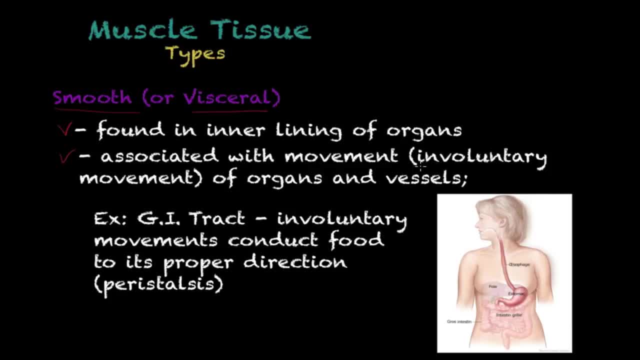 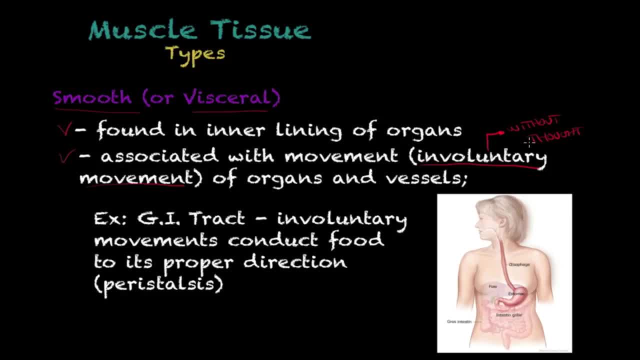 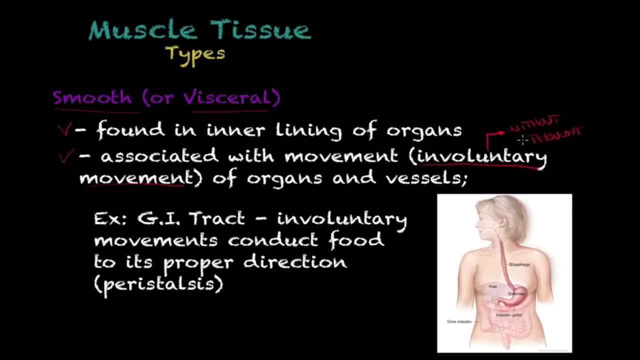 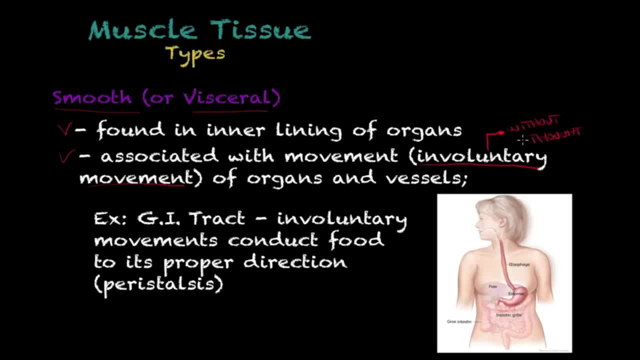 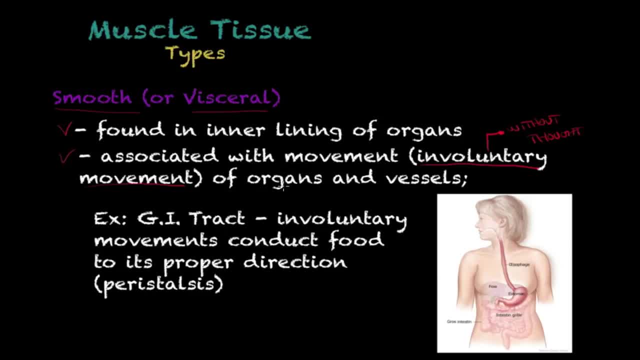 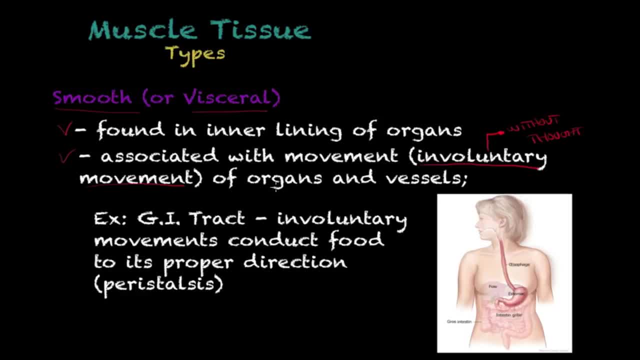 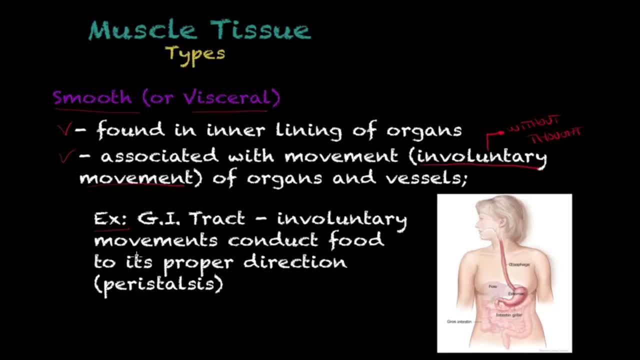 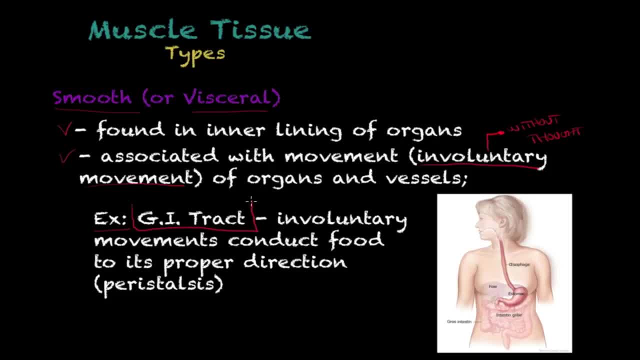 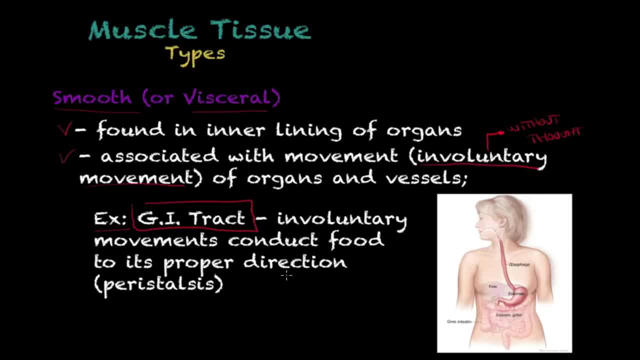 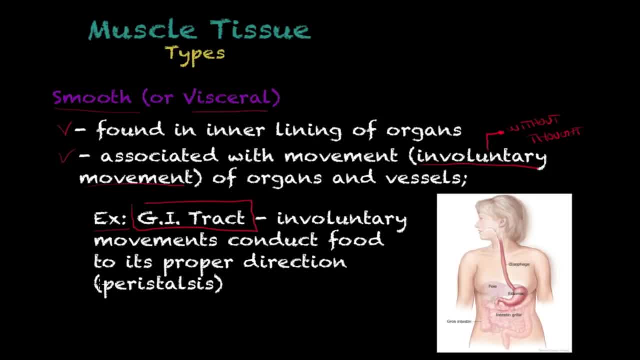